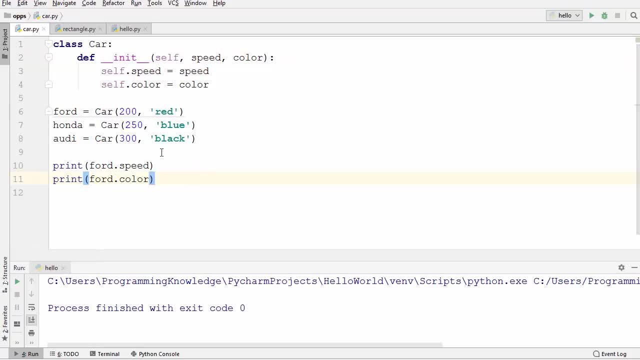 Now let's say we want to change the value of speed. So if you want to change the value of speed, you can simply take your object, for example, forward, dot your attribute name, for example speed, and then you can directly change it. for example 300. And when I run the program it's going to print the new speed, which is 300.. Initially we have set the speed to 200.. In here we can also put, let's say, the speed as string. 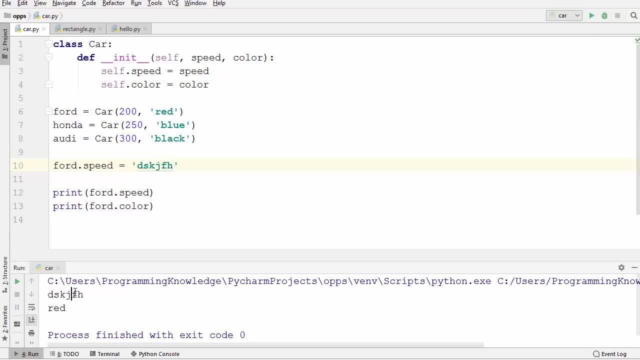 Which is very stupid, but will it work? It works, you can see here, And this can break the function in which the speed is used. So therefore, it is very important that we protect our data and only give the access to our data to the other users. So encapsulation is particularly important when you want to give your code to some other people, because they might want to change your code. So let's see how we can. 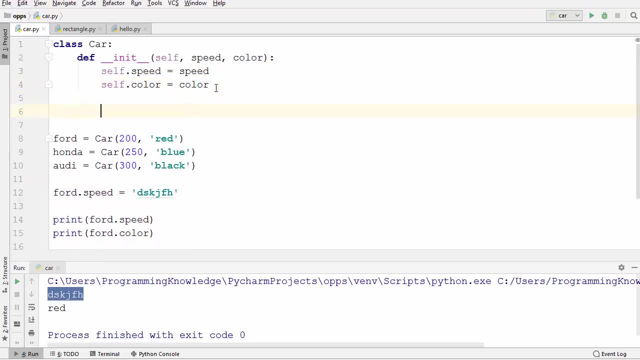 encapsulate our code. So to encapsulate our code, we create functions. So let's create our first function, which is to set the value of speed. So I'm going to just say set underscore speed And inside the parentheses it's going to take self as the first argument, which is the default, And second is the value of speed. So so I can say value here, right, And then, once we have the value of speed, we can set the value of speed. 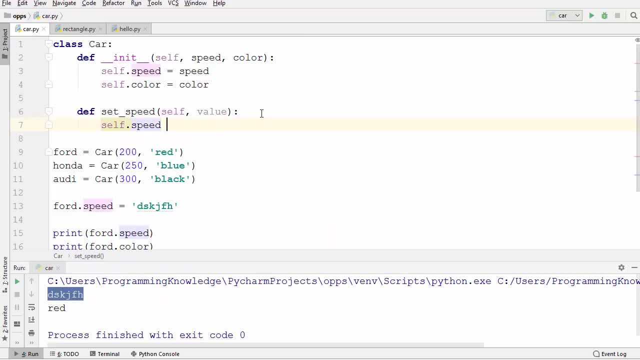 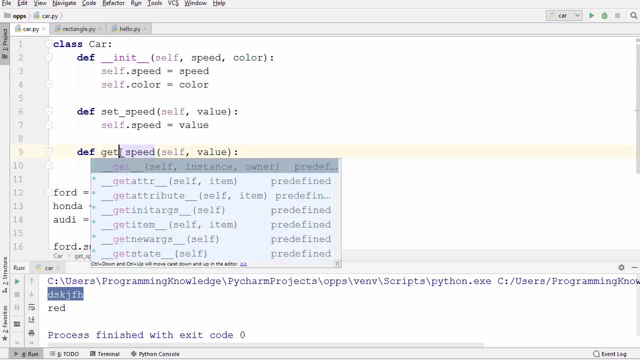 We can just call self dot. speed is equal to value. Similarly, we can create a get method for the speed. So right now we have created the set method to set the speed And now we are going to create a get method to get the speed. And in order to get the speed, we don't need to pass any argument, we just need to return this speed which is already set. So we can just write return. 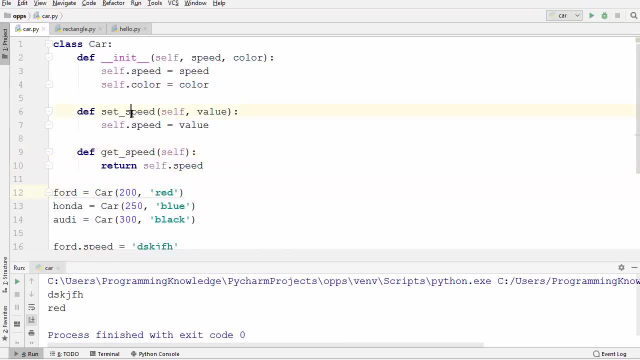 And then self dot speed. So we have created two functions: set and get. these are also called setter and getter for the attribute which is speed in our case. So let's use these functions instead of this kind of setting of data. So first of all, I'm going to call this forward object dot set speed method out of this object, And then I'm going to pass the new speed using this set method Now in order to get this. 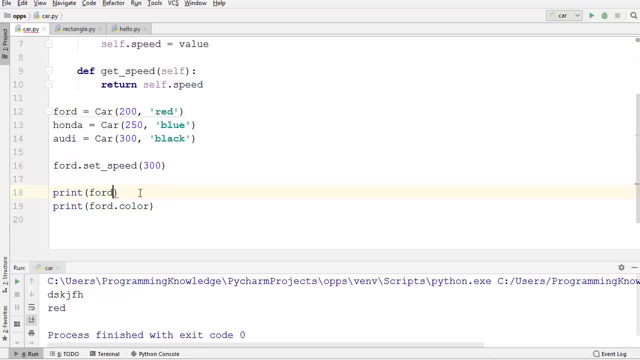 speed I can write. instead of this forward dot speed, I can just write the forward dot get speed, which is going to give me the speed of this forward object. So I'm going to run the code And you can see it prints the speed which we have set using the set method. But still, will this protect your data? Let's see. So I'm going to once again try to use forward dot speed And then 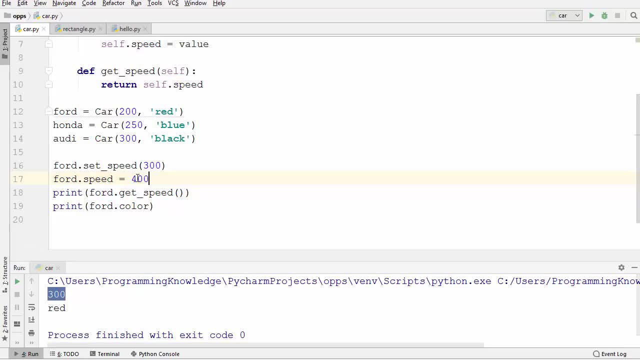 I will try to set the new value of speed. Will it be a problem? No, So you can see when I try to get the speed. the new speed is set, And we want to prevent this kind of setting of data using this equals to symbol, So we need to somehow make our attribute private. Now, if you are familiar with other object oriented programming languages like Java or C++, they use the 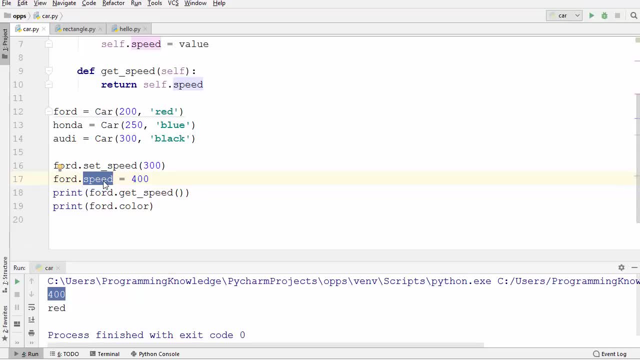 keywords like public, private or protected in order to mark their attributes or the member variables as the private or public or protected. But Python doesn't have any of these keywords. So how we can make our data private? So let me give you first of all an example. So I'm going to go to this class which is hello, And here I'm going to set some values. So first value is, for example: 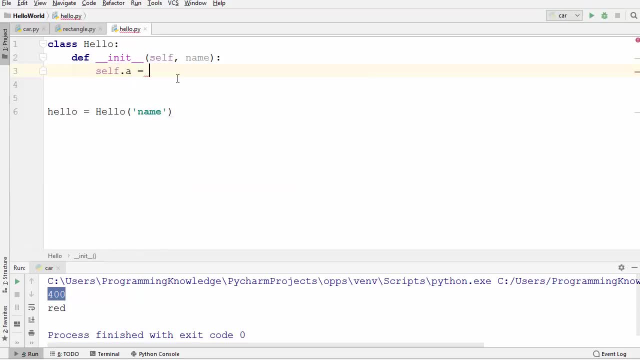 self dot a is equal to 10.. Second value is self dot underscore B is equal to 20.. And the third value is self dot underscore underscore C is equal to 30. So we have created three member variables in this hello class. One is a, second is underscore B and the C is with two underscores. 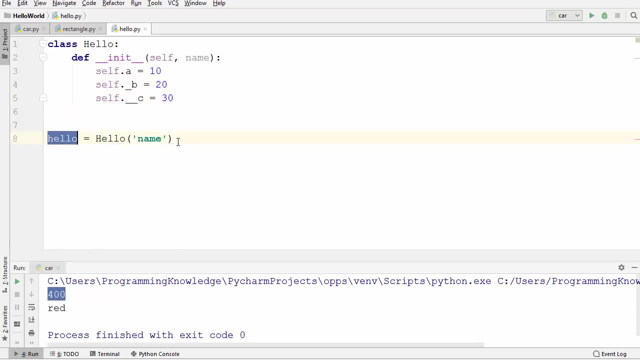 so this has private consists in front of it And let's try to access all these three values. So I'm going to just use print method and then the hello object dot a, And similarly I will use this print to get the value of Underscore B. 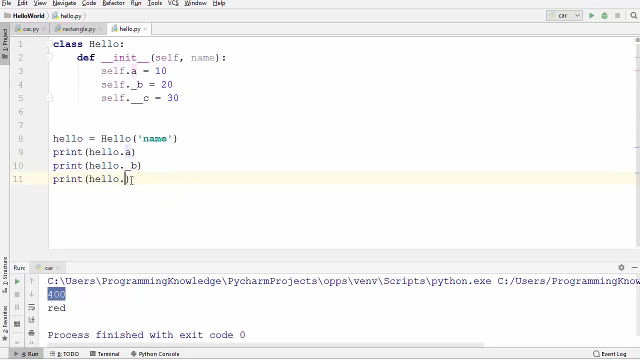 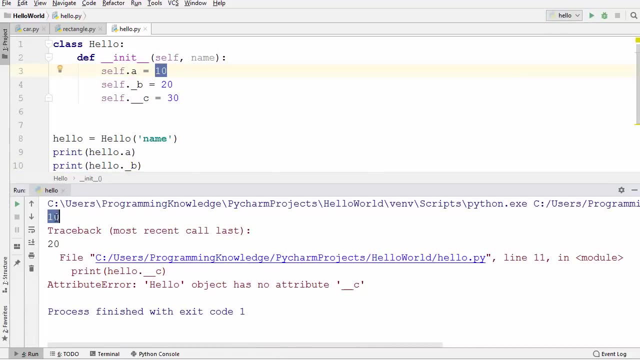 and also dot underscore, underscore C, And let's try to run se And let's see what happens. And you can see that, alltså, here the first value which is printed here is 10, which is the value inside the a variable. so this: 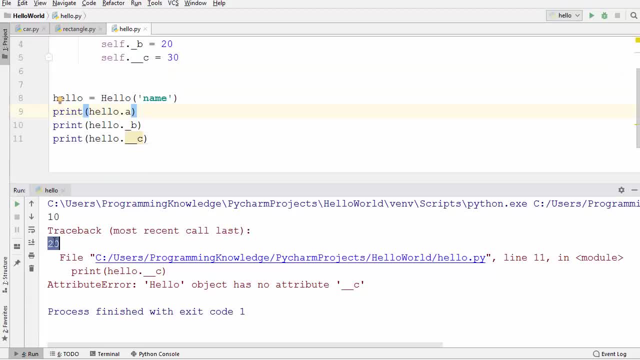 code was executed successfully. now we can see here that 20 is also printed. that means this code is also executed successfully. but at the time of underscore, underscore c, when we want to use this underscore, underscore c, outside the class, it says: hello. object has no attribute called. 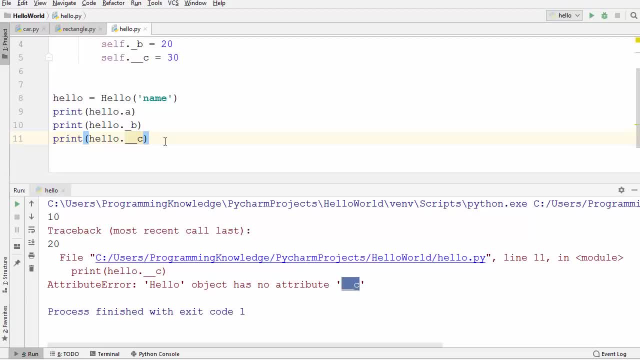 underscore, underscore c, and this is the point. so underscore, underscore you can use to make your attribute private. okay, so this is a convention. there is no keywords like private in python. that's why python uses this kind of convention in which, whenever you use double underscores, it makes your data private. when you use single underscore, that also means that it's 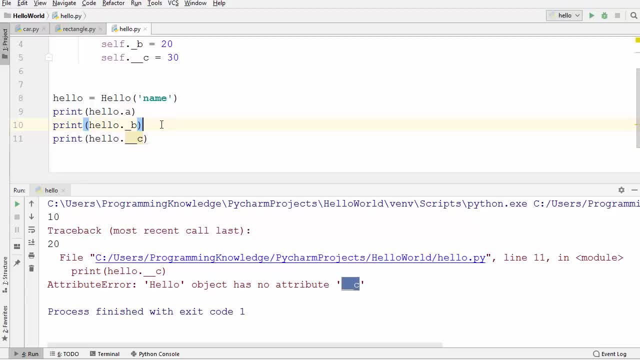 a private variable, but this is only a convention. nothing stops you to change the value of underscore b or accessing the value of underscore b. okay, so if you truly want to make your data private, then use double underscore in front of your variable. when you use single underscore, that means it's a partially private. 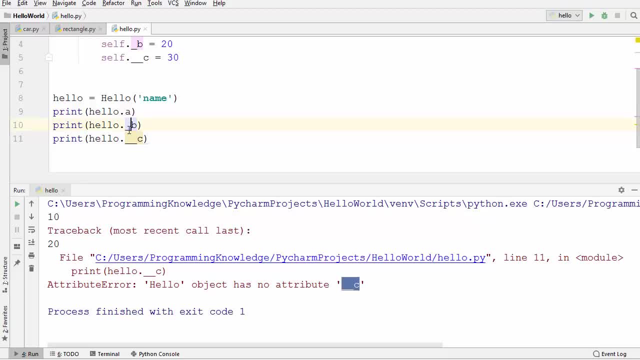 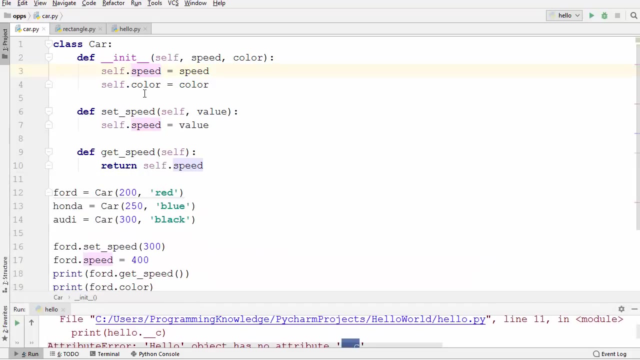 variable and it's only a convention. okay, so let's go to our car class once again. and now we know that we can add double underscore in front of our variable name. so we have two variables here. one is speed, so let's add double list underscore in front of speed and also let's add double underscore in. 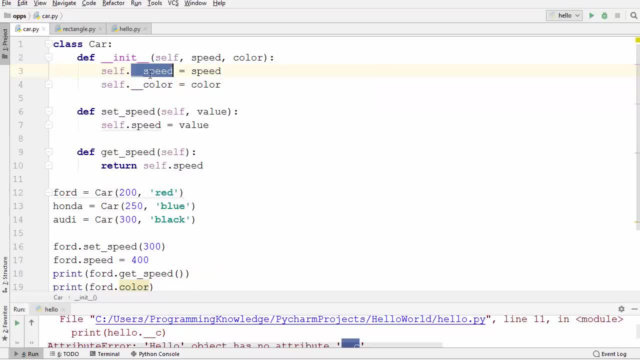 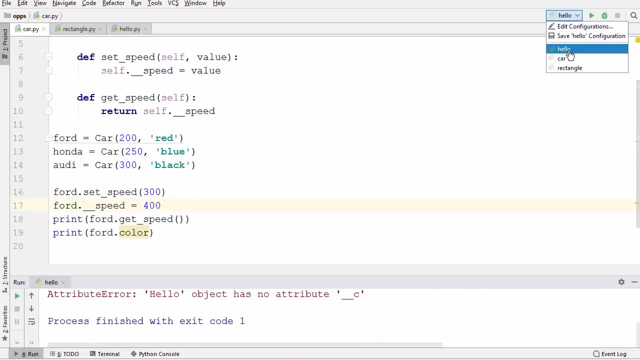 front of this color variable to make both of them private. so i'm going to change this value of speed in getter and setter also, and now let's try to access this value using this ford object which is underscore- underscore: speed. now let's try to run our program. so i'm going to change the file and 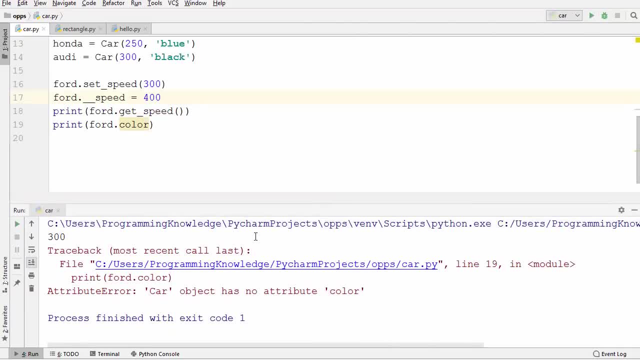 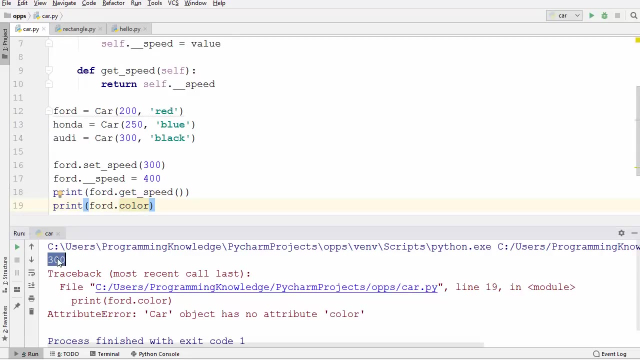 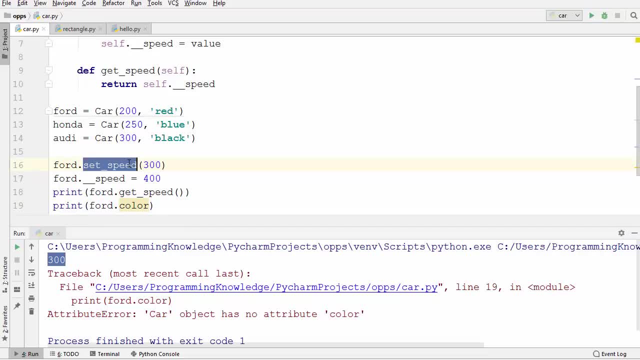 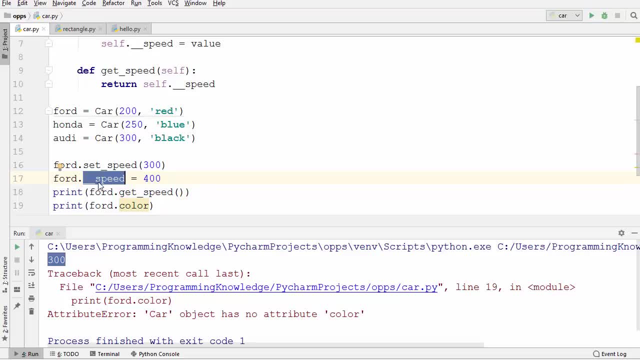 change the speed using this underscore- underscore variable, because now it's a private variable and that means we cannot change the value using this variable. we need to use this set function in order to change the value of the speed also, if you want to use this underscore underscore color. 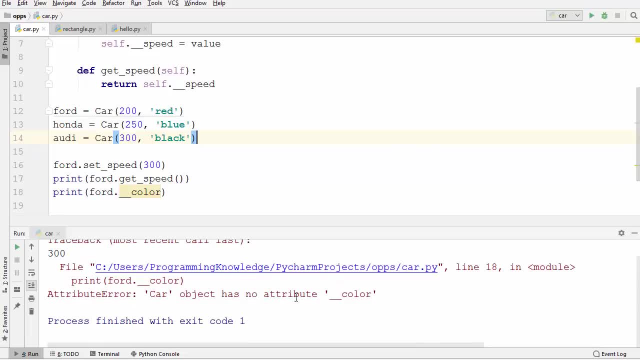 here and let's run the code. this will also give you an error, because this underscore- underscore- color is private. so either you can remove this code or you can create the setter and getter method for the color also. so let's create the setter and getter method for the color. 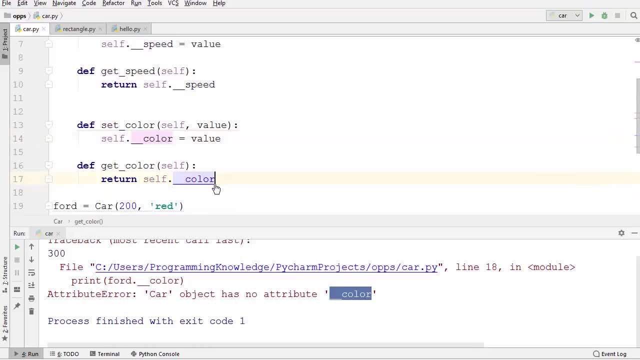 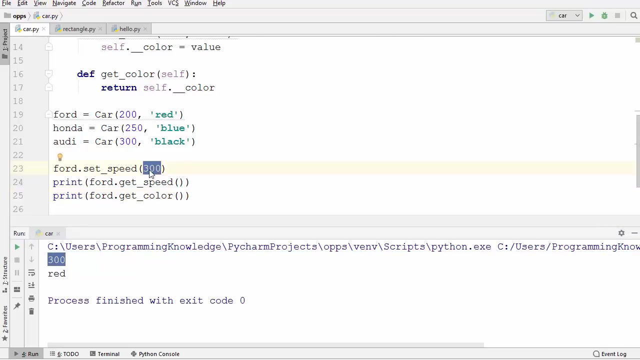 and now we can access the value of color using the get color method. right? so instead of this get speed, we can just write 4 dot, get color and it's going to give us the value of color. and now you can see that there is no error. and the speed here is 300, which we have set. 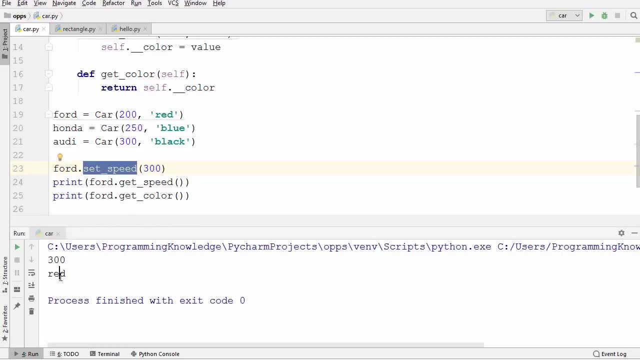 using this set speed method and the color is red, which is the color we have given using this argument in the constructor, and this type of restricting your data access using functions is called encapsulation. let's do the same thing with our rectangle class also and let's create the setter and getter method inside the rectangle class. so you already know we can.